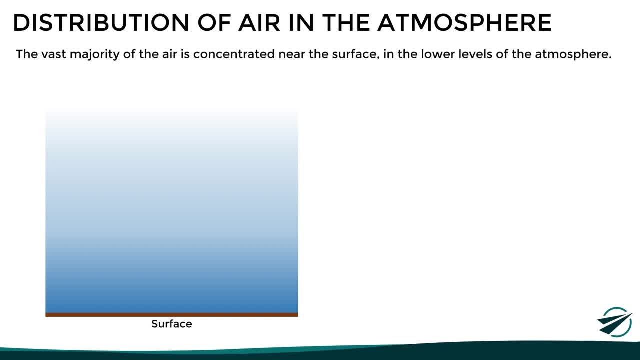 This implies that, due to the Earth's gravity, most of the air is concentrated near the surface, in the lower levels of the atmosphere. This way, 50% of the air that constitutes the atmosphere is concentrated within the first five kilometers of altitude. 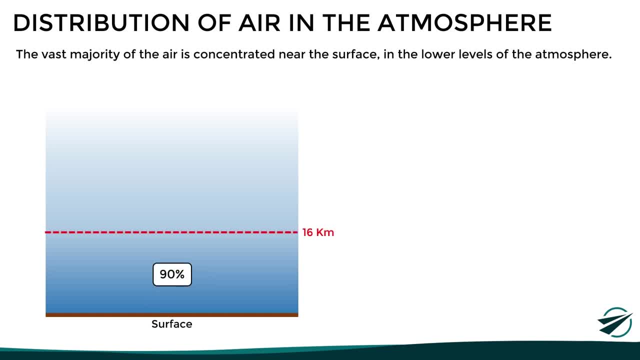 90% of the air is concentrated within the first 16 kilometers and 99% of the air is below 32 kilometers of altitude. With this, it is evident that, as the altitude increases, the air becomes less and less dense. However, despite the fact that below 32 kilometers of altitude we find 99% of atmospheric air, 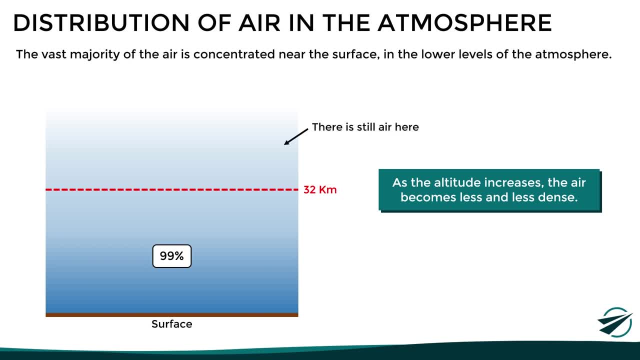 the truth is that above this level we still find molecules of air, but they are very, very spread apart. So at this point you might be wondering: where does the atmosphere end, Or in other words, what is the altitude at which we find the boundary between atmosphere and space? 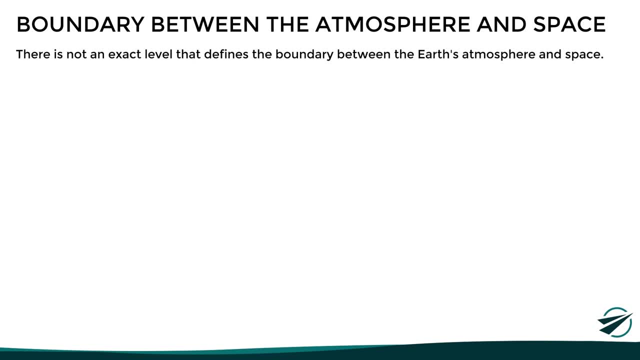 Well, actually, there is not an exact level that defines this boundary. This is because, as we go up in the atmosphere, the air gradually becomes less and less dense until we eventually reach space. However, from an aeronautical perspective, the Karman line is often: 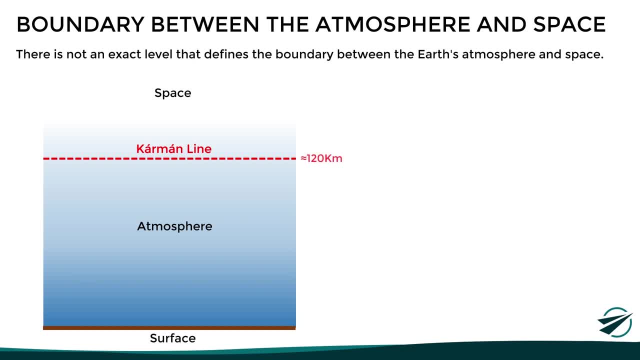 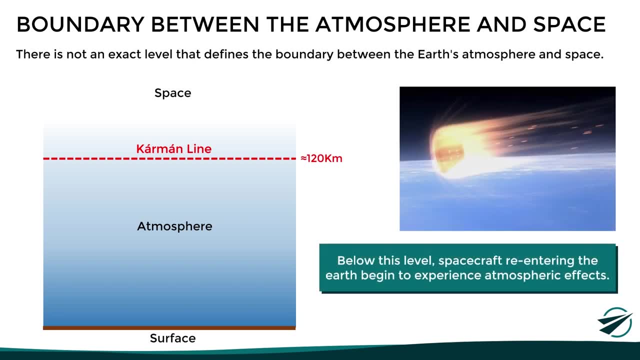 used as reference to the position of the atmosphere and therefore is often used as reference to the reference for this, which is at an altitude of approximately 120 kilometers. Using this line is useful because, below this level, the spacecraft re-entering the Earth begin to experience. 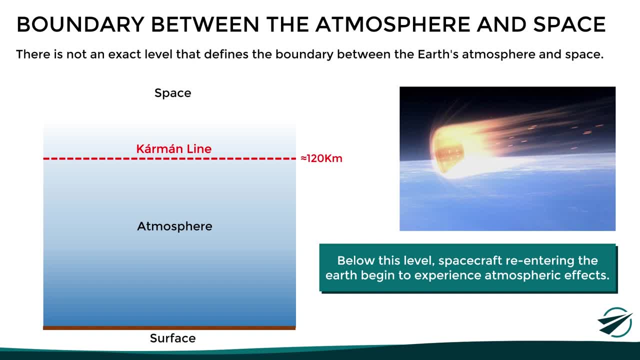 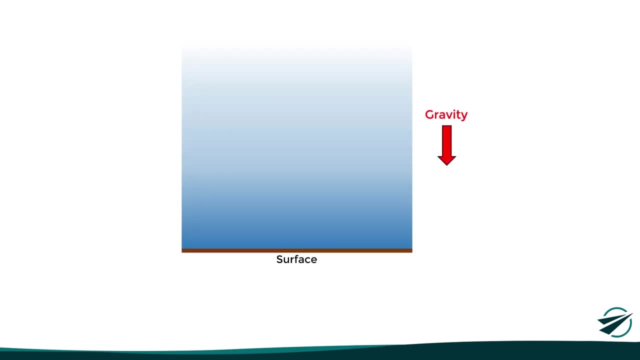 significant atmospheric effects. However, we must clarify that above this altitude we can still find air, but it is so widely spread apart that in practice, it does not have any significant influence on larger objects. Now, in this order of ideas, we could think that, due to the Earth's gravity, 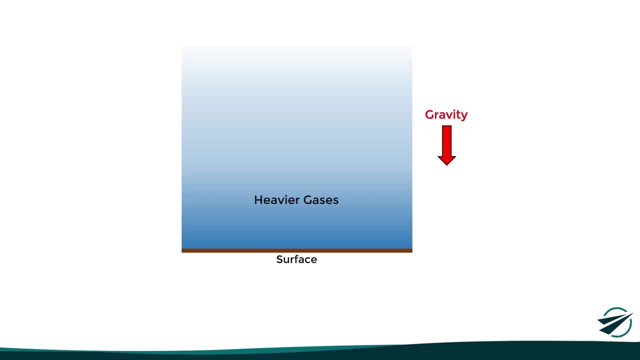 in the lower levels of the atmosphere, we would find the heavier gases, such as oxygen or carbon dioxide, while in the upper levels we would find the lighter gases, such as helium or hydrogen. However, the truth is that, in practice, this just does not happen. This is because the Earth's 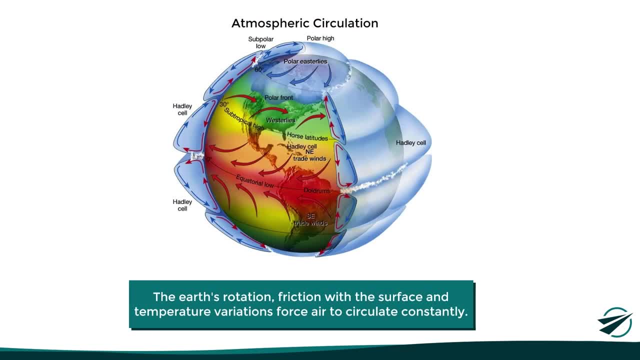 rotation, the friction with the surface and the temperature variations force air to circulate and mix constantly, which is known as atmospheric circulation. This constant atmospheric circulation in search of equilibrium, especially at low levels in the atmosphere, causes the gases to mix with each. 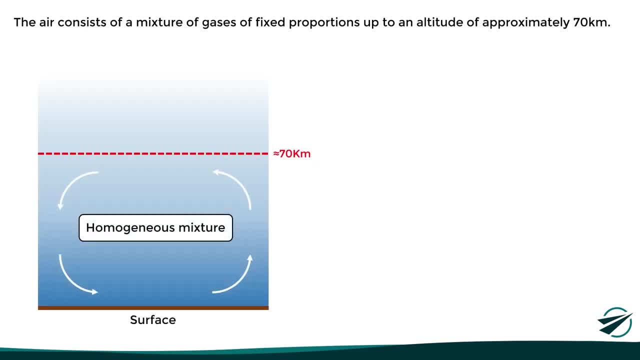 other. This way, we obtain a mixture of gases of fixed proportions from the surface up to an altitude of about 70 kilometers. Above this level, the atmospheric circulation is not as significant. so at higher altitudes, gases begin to separate due to gravity, according to the weight of each. 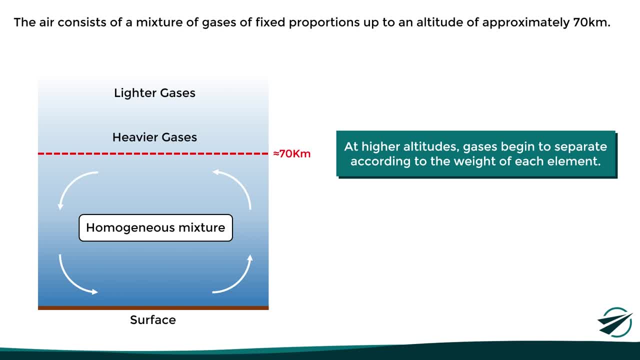 element, leaving the heavier gases at the bottom and the lighter gases at the upper levels. With this being said, since air operations are carried out in the lower levels of the atmosphere, let us look at the composition of this mixture of gases found near the surface. 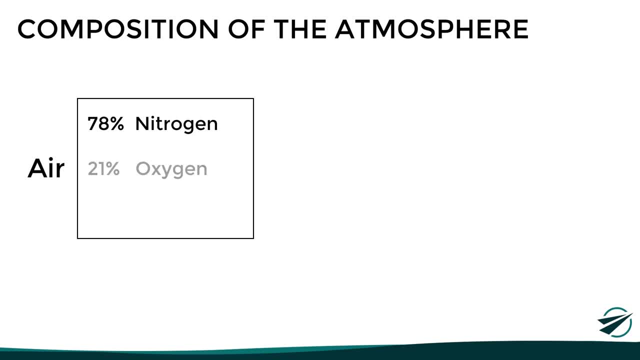 The air here is composed of 78% nitrogen, 21% oxygen and 1% of other gases such as argon, carbon dioxide, neon, helium ozone and others. It is important to note that, since we are in the 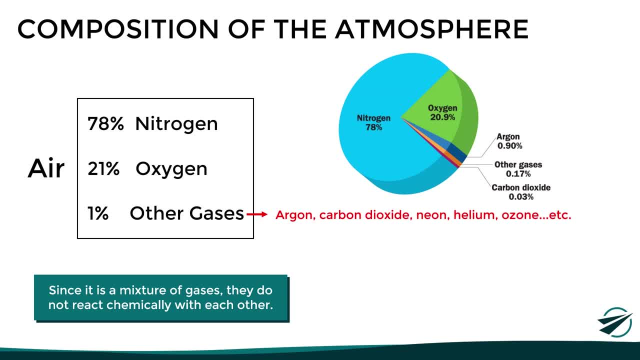 middle of the atmosphere. we are talking about a mixture of gases. it means that they do not react chemically with each other, maintaining their original form as inner gases. Now, we must emphasize that this is the composition of a dry sample of air under ideal conditions. 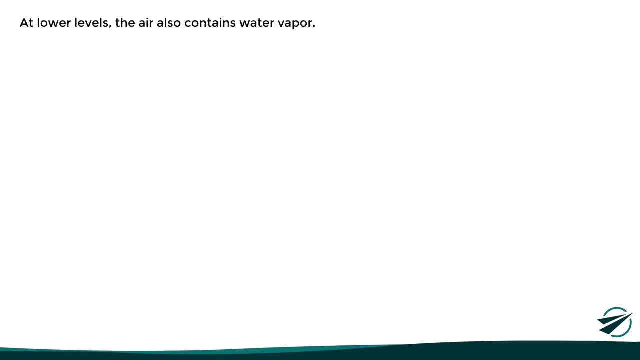 Because, in practice, in the lower levels of the atmosphere, the air also contains water vapor, which is known as humidity. Water vapor is simply water in its gaseous state and therefore humidity is the measurement of how much water vapor is contained in the atmosphere. 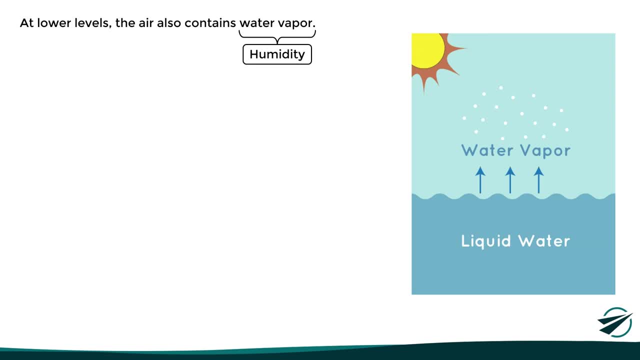 To get an idea of how significant its presence is. the water vapor content in the atmosphere at sea level normally varies between 0 and 5%, depending on factors such as air temperature or the geographical characteristics of the area. Now, since humidity depends in part on the air temperature, as we go up in the atmosphere and the air temperature decreases, the humidity also decreases, so that above an altitude of 10 kilometers, the temperature of air in the atmosphere decreases. 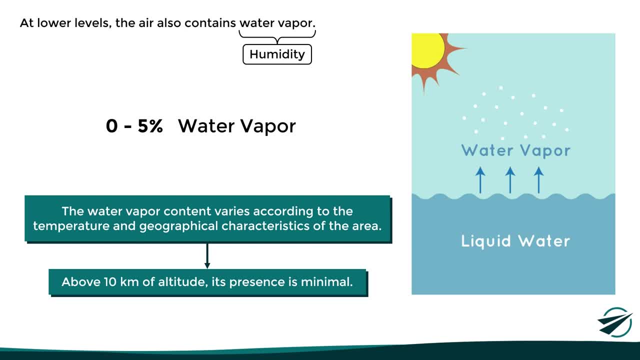 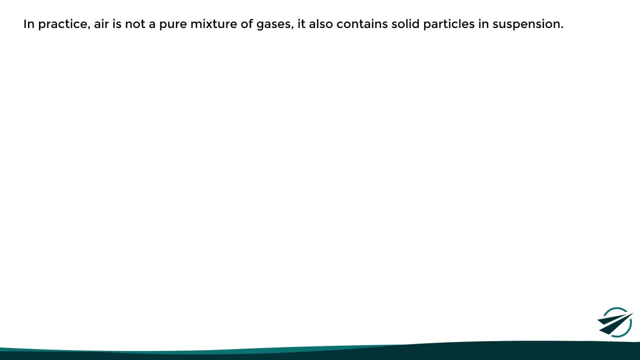 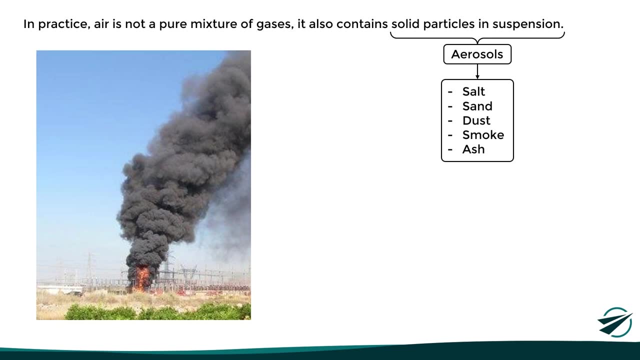 launders, the presence of water vapor is minimal. Now, in practice, apart from water vapor, the air also contains tiny little solid particles in suspension, known as aerosols. Here we can highlight things like salt, sand, dust, smoke and ash, And even though in many cases these aerosols 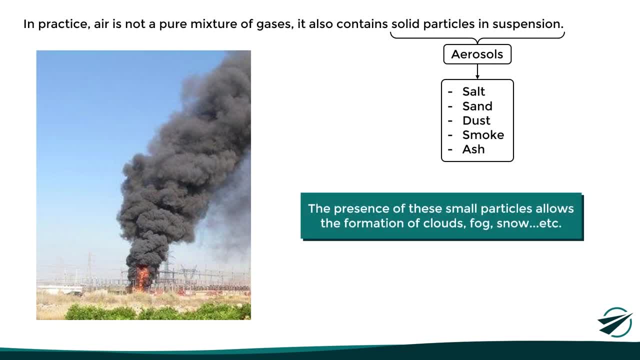 are invisible to the naked eye. their presence in the atmosphere allows the formation of clouds, fog, snow, among other meteorological phenomena. This is because these tiny little particles act as condensation and freezing nuclei, but we will talk about them in more detail in a future video. 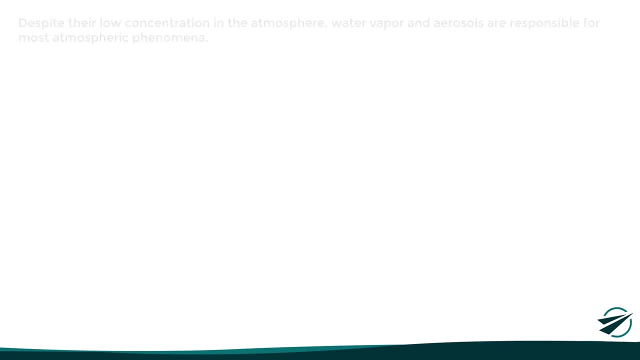 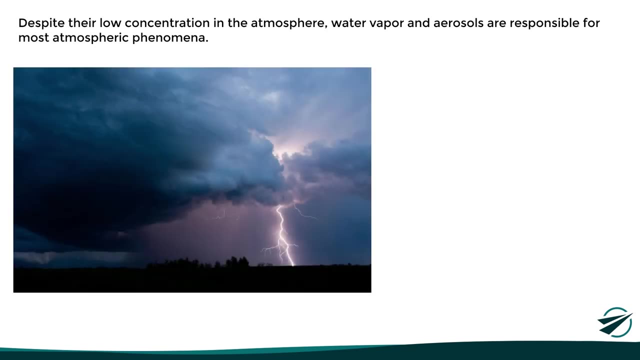 Now, as we just said, despite their low concentration in the atmosphere, water vapor and aerosols are responsible for most atmospheric phenomena. Actually, the study of the vast majority of meteorological phenomena is based on the analysis of the behavior of water in the atmosphere, whether it is in liquid, solid or gaseous state. 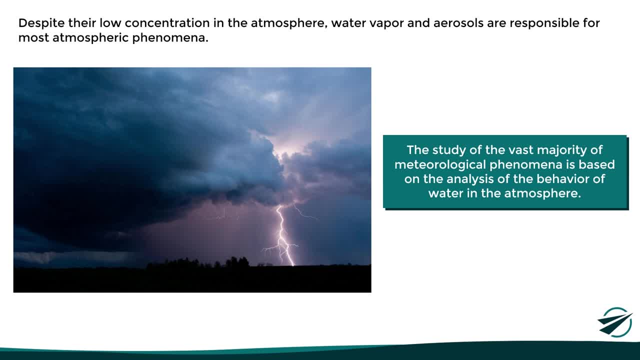 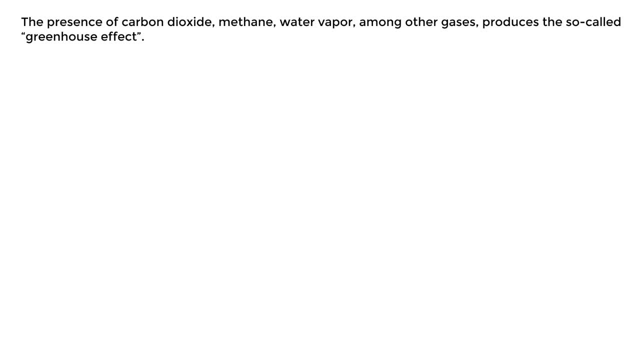 However, although they contribute substantially, these are not the only factors that condition the Earth's climate, as there are also those known as greenhouse effect gases. Here we can highlight carbon dioxide, methane or water vapor, which allow us to have adequate and pleasant 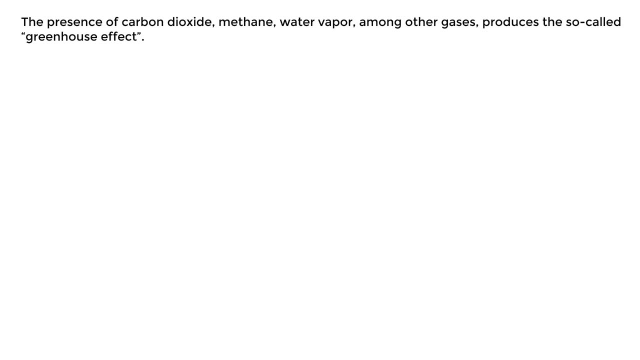 temperatures for the evolution of life and ecosystems. Let's take a look at a quick explanation of what the greenhouse effect gases are. During the day, the sun emits short-wave radiation that is absorbed by the Earth's surface, causing its temperature to rise. This type of radiation passes through the atmosphere easily. 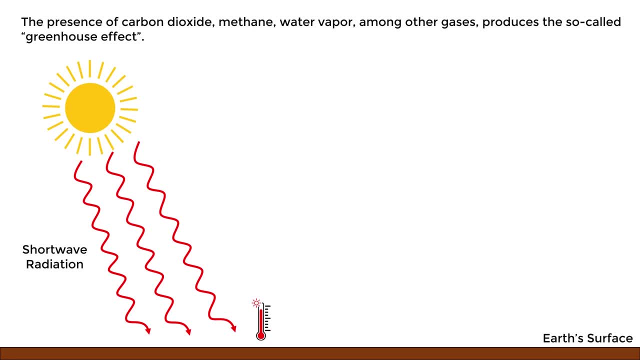 as it is not absorbed by the gases that constitute the air. However, during the night, the hot surface emits long-wave radiation back into space, but on its way, this type of radiation is absorbed by some gases in the atmosphere, specifically the greenhouse gases. 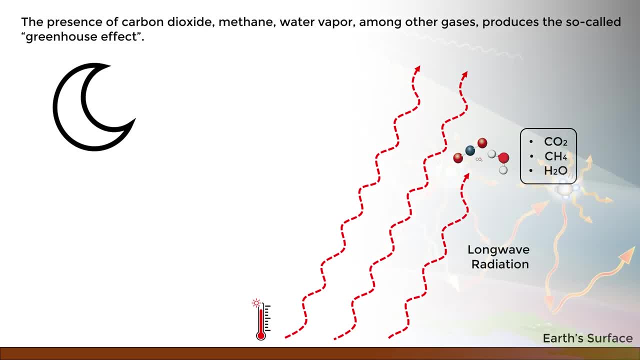 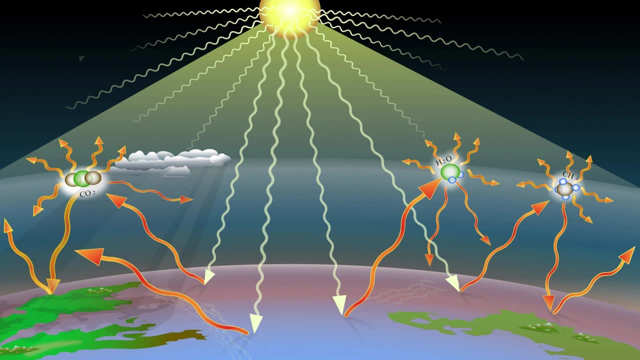 This effect prevents all the heat from being lost back into space, since some of it remains trapped in the atmosphere, allowing temperatures to be suitable for life. Now it is important to clarify that this greenhouse effect is necessary to maintain the natural balance of the planet. to a certain extent, The problem is when there is an excess. 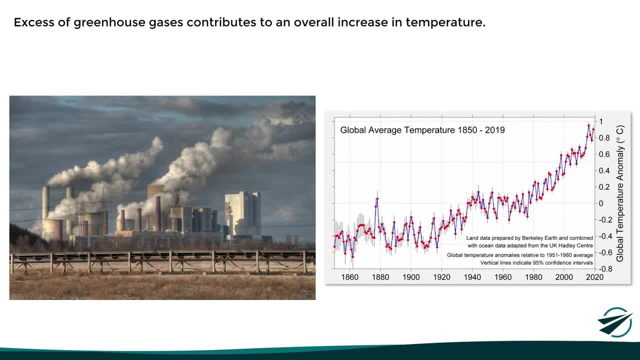 of these greenhouse gases, as this necessarily leads to a general increase in global temperatures. This phenomenon is known as global warming, and it can generate significant climate changes, among other negative effects on ecosystems, but we will not go into detail on this topic in this video.